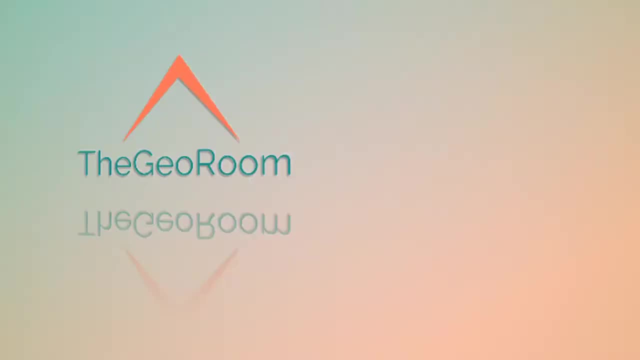 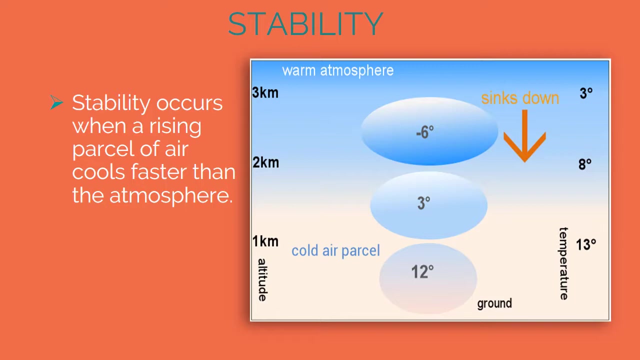 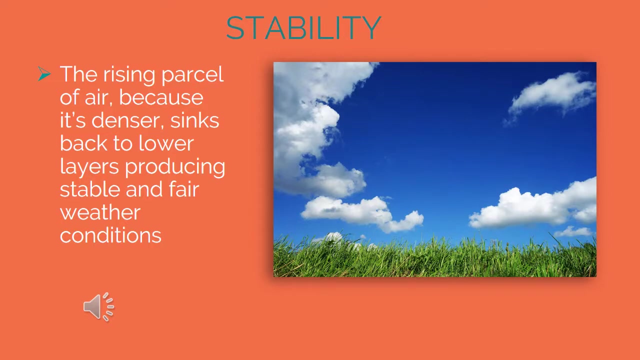 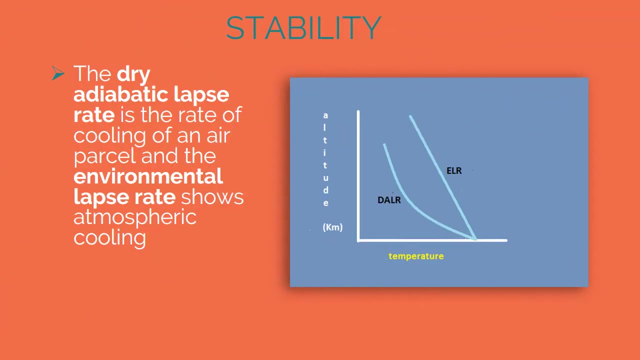 Stability. Stability occurs when a rising parcel of air cools faster than the atmosphere. The rising parcel of air, because it's denser, sinks back to lower layers, producing stable and fair weather conditions. The dry adiabatic lapse rate is the rate of cooling of an air parcel and the environmental lapse rate shows atmospheric cooling. 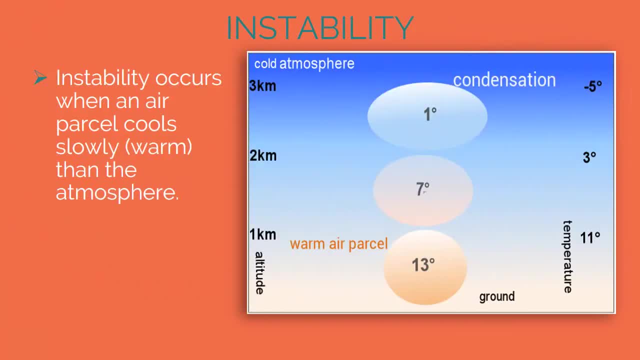 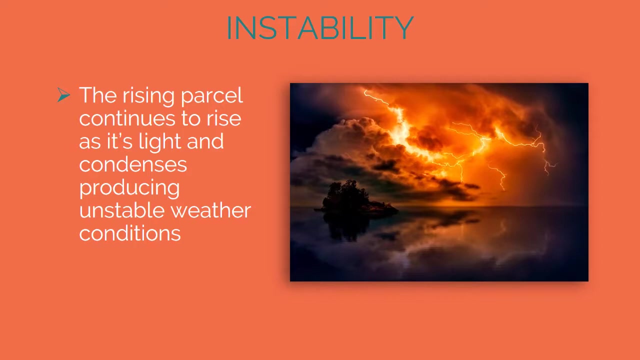 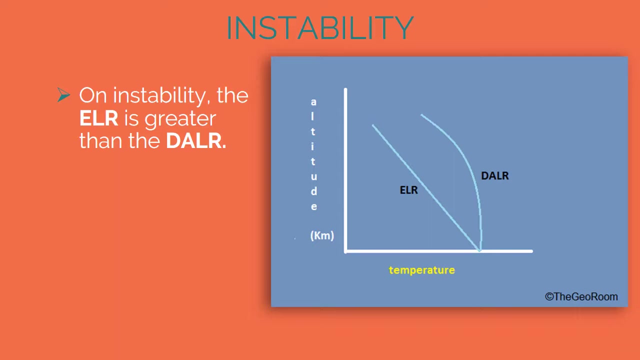 Instability. Instability occurs when an air parcel cools slowly than the atmosphere. The rising parcel continues to rise as its light and condenses, producing unstable weather conditions. On instability, the environmental lapse rate is greater than the dry adiabatic lapse rate. 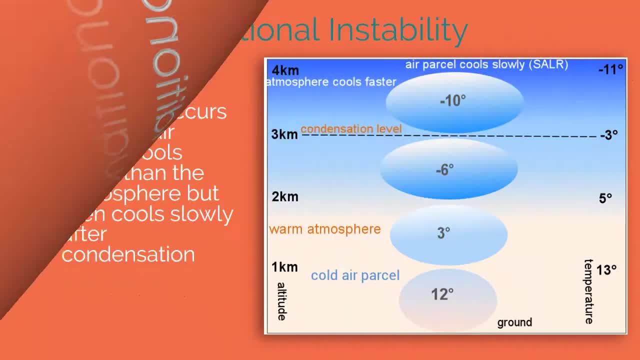 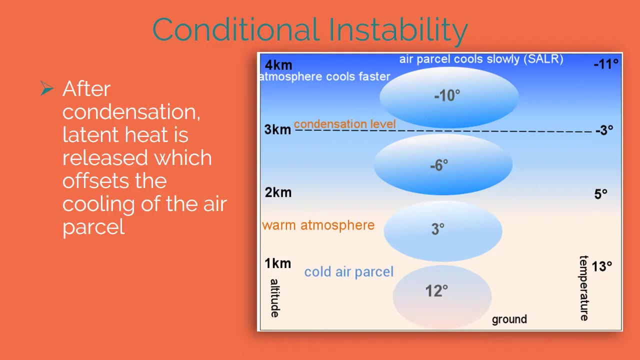 Conditional instability. Conditional instability occurs when an air parcel cools faster than the atmosphere, but then cools slowly after condensation. After condensation, latent heat is released which offsets the cooling of the air parcel. The air is unstable because it has risen to condensation level in the first place. 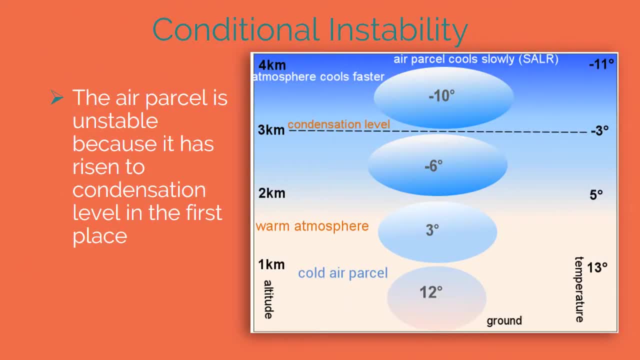 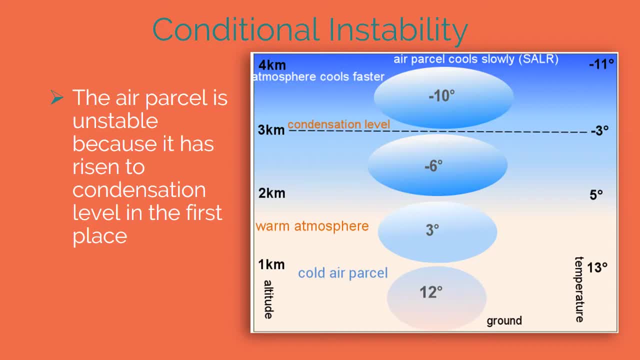 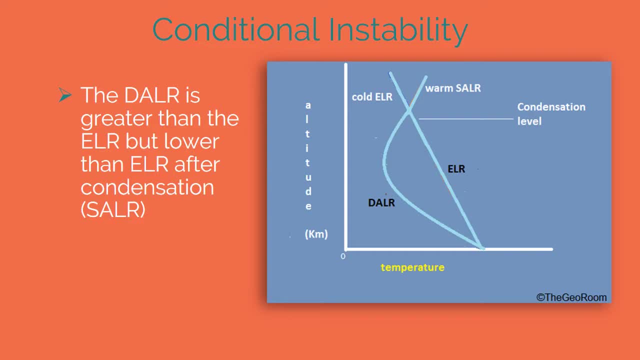 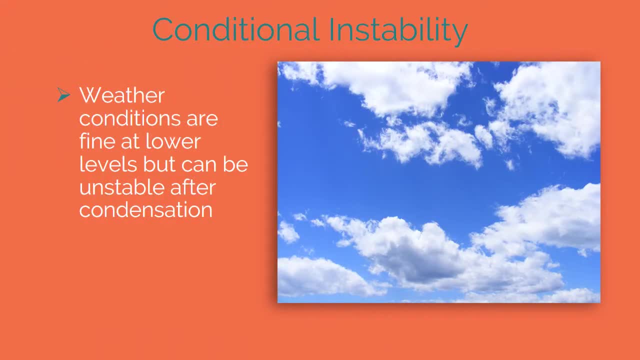 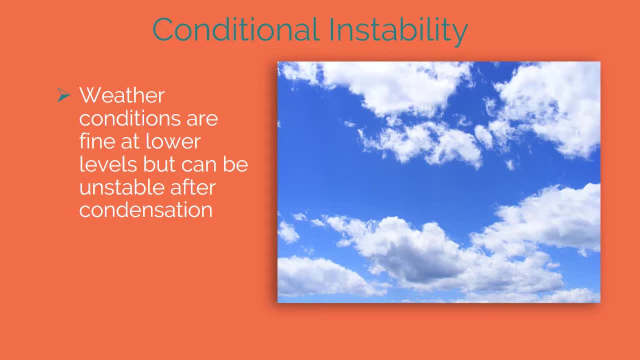 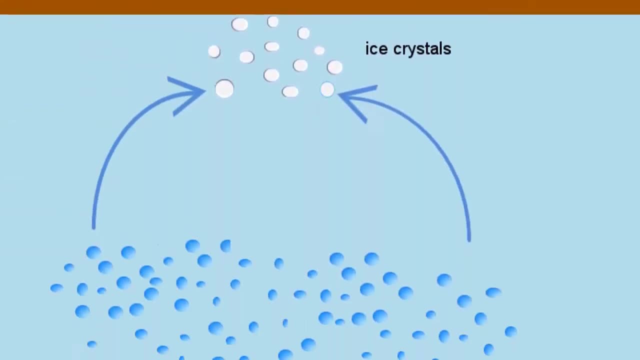 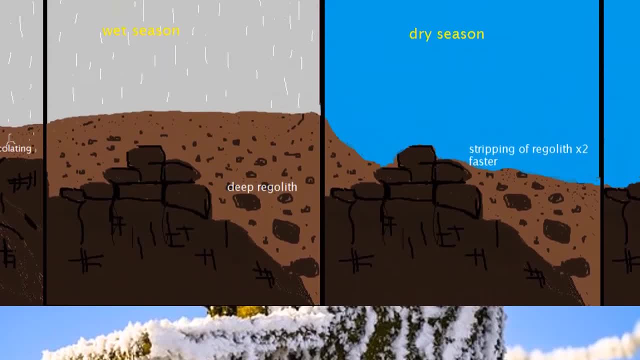 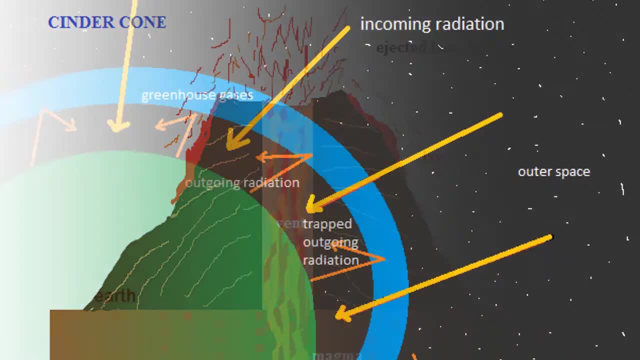